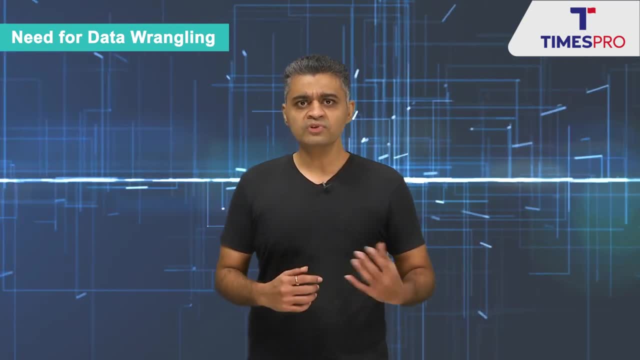 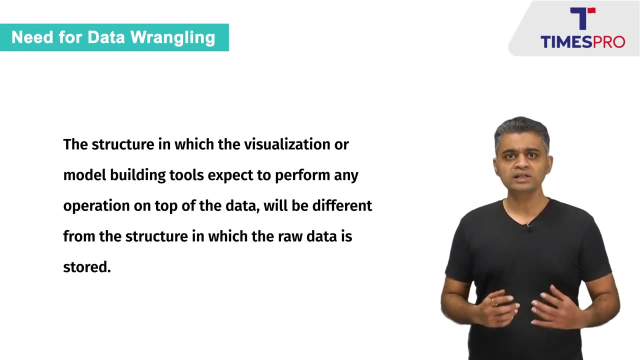 We read the raw data using various tools to either visualize or build models. The structure in which visualization or model building tools need the data to perform any operation will be different from the structure in which the raw data is stored. So let us start with the raw data. 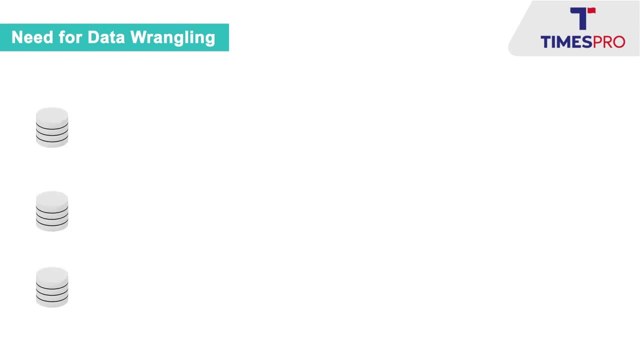 The process or the steps that are used to convert the raw data from its original structure to the structure that is expected by these tools is called as data wrangling. There are multiple data wrangling techniques that are widely used. depending on the requirements, We might use one or multiple of these techniques. 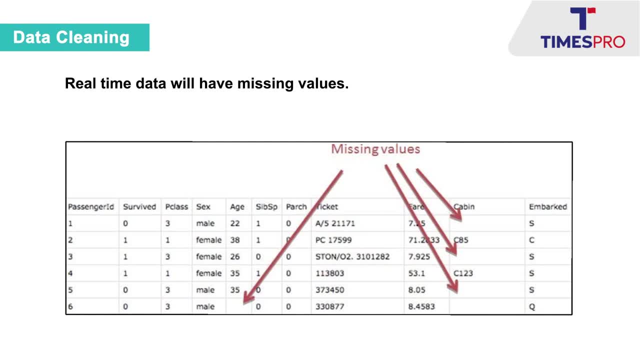 Most of the real-time data will be having missing values, but many machine learning algorithms do not take data from the original data, So let us start with the raw data. We need to treat these missing values properly before we build any machine learning model. 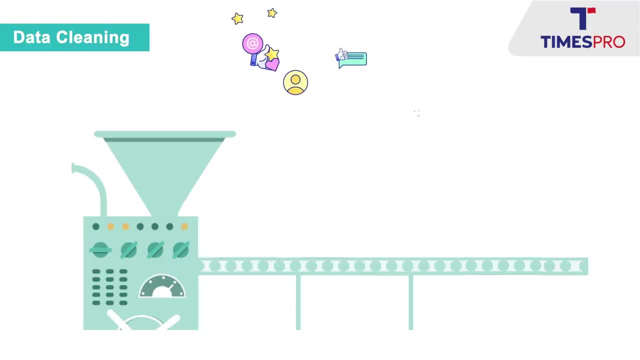 Next comes the text data cleaning. If our data contains any text column, especially the data that comes from social media platforms or scraped from websites, or data that is manually entered through web forms, it will have a lot of text columns with informal language. These informal texts might be easy to understand. 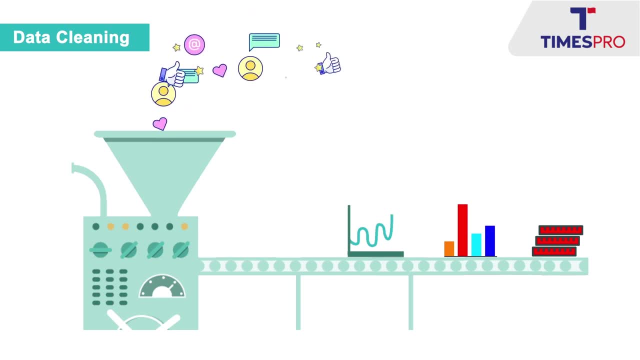 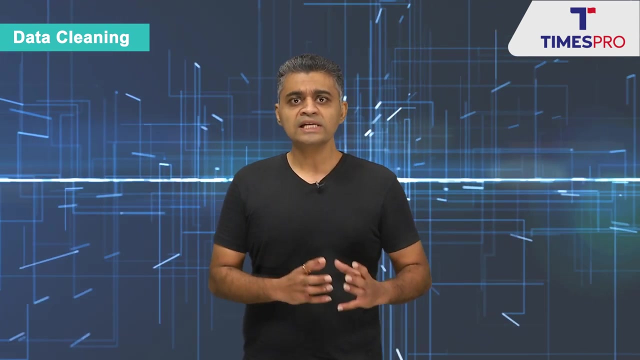 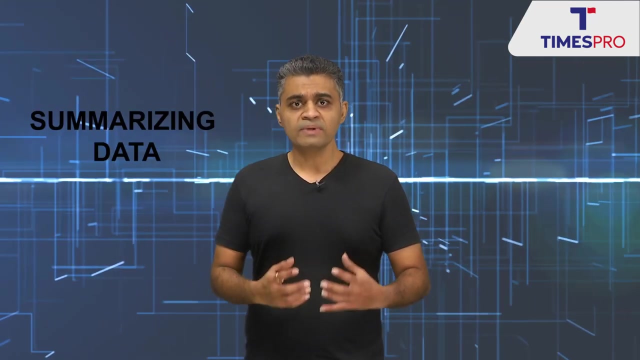 But it is very difficult for computers and algorithms to interpret These text. data fields require a lot of cleaning. Apart from these, there are many broad data quality issues you will encounter while cleaning the data. The next data wrangling operation, which very often that we will be using, is summarization. 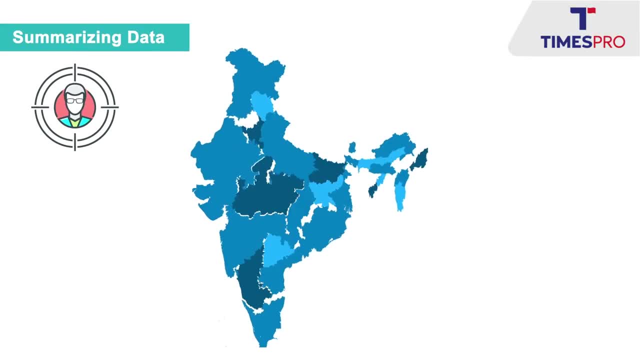 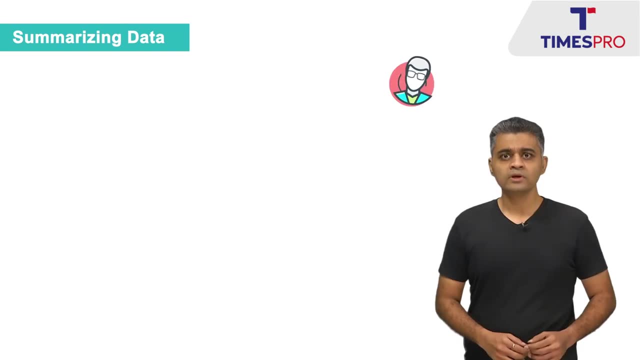 Let us say a company CEO wants to identify the top data column that is being used to clean the data. In this case it is the top 5 cities in which sales went down for the last 3 years consecutively. To calculate this information, one has to hit the sales database table, which will have 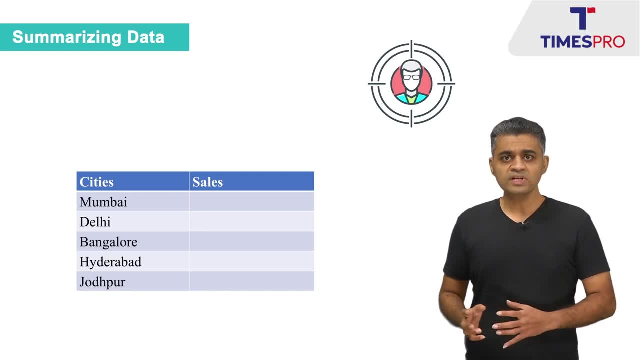 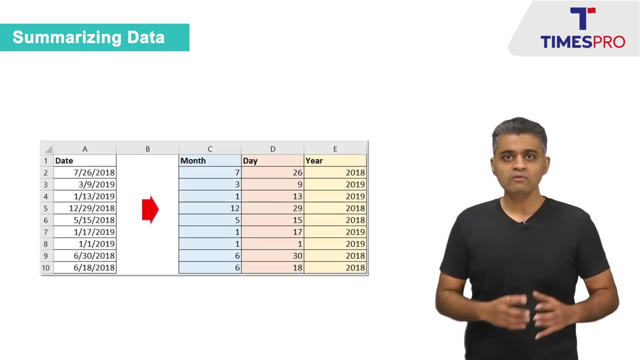 sales values from different cities, And these tables will have day-wise sales across the city, But what we need is yearly sales, So we need to convert the data from one granularity, that is, from day-wise, to another granularity, that is, to year-wise.